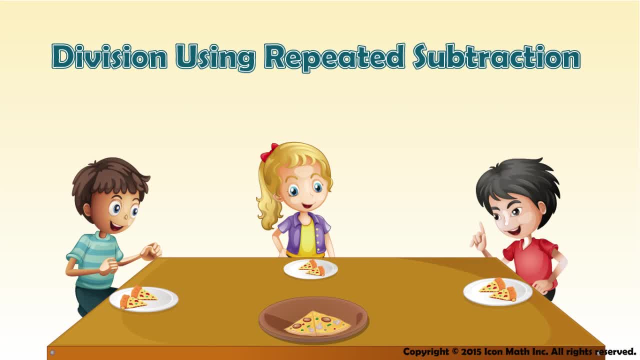 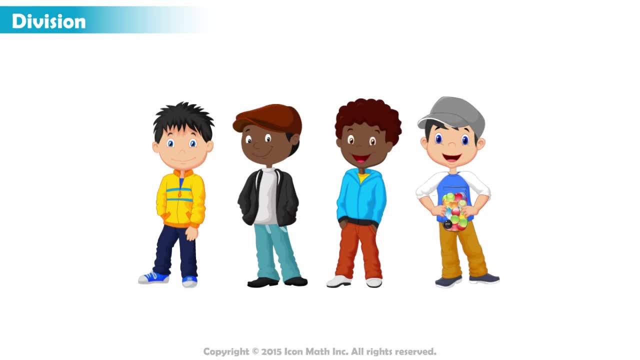 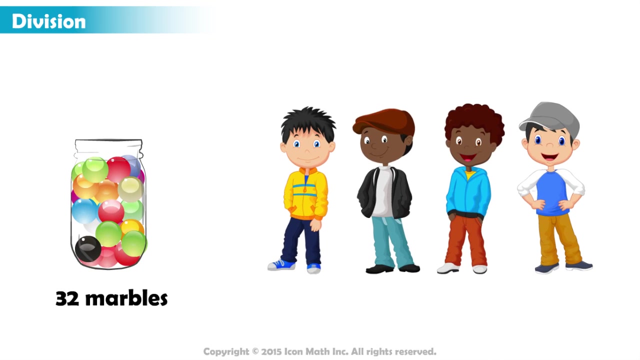 DIVISION USING REPEATED SUBTRACTION. Jim is going to shoot marbles with his friends. To start the game, each player must have the same number of marbles. Jim has a total of 32 marbles and he's playing with three other friends. 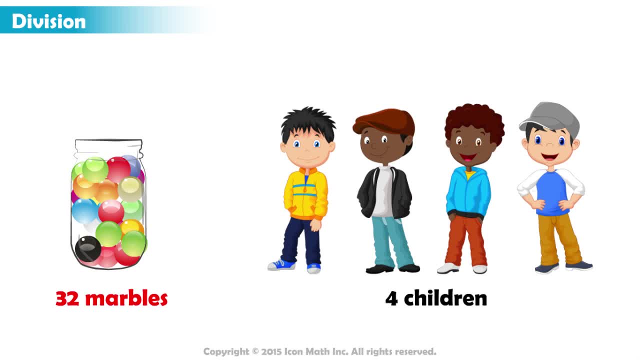 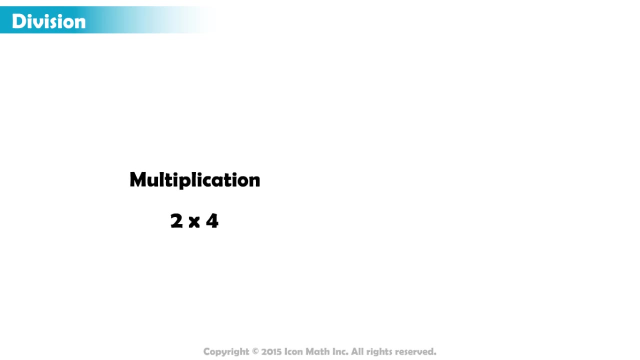 So if Jim divides the 32 marbles among the four people- him and his friends- how many marbles would each person get? Remember how multiplication is just a shortcut of doing repeated addition. Similarly, division is about doing repeated subtraction. So if we have 32 marbles and there are a total of four people each waiting to get some marbles, 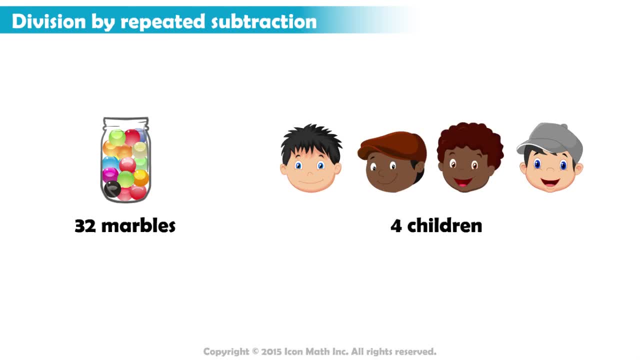 how do we do the repeated subtraction? Since 32 is the total marbles we have, it is the dividend and 4 is the divisor, because they are the people who divide the marbles. So if we have 32 marbles and there are a total of four people each waiting to get some marbles, 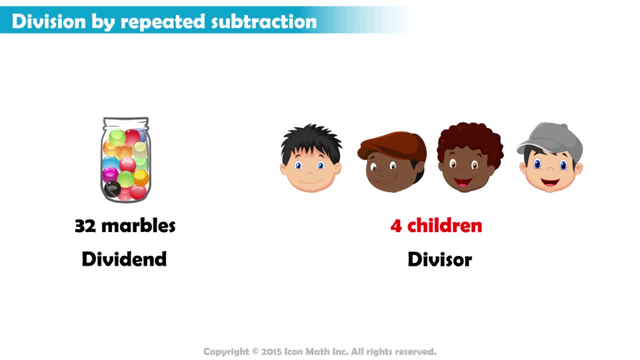 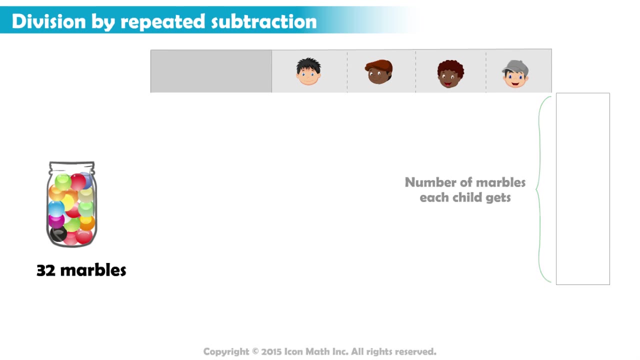 we are the people among whom we want to divide the marbles. To carry out this division by repeated subtraction we draw a margin so that we keep track of how many times we gave away marbles. So first we take away four marbles from 32,. 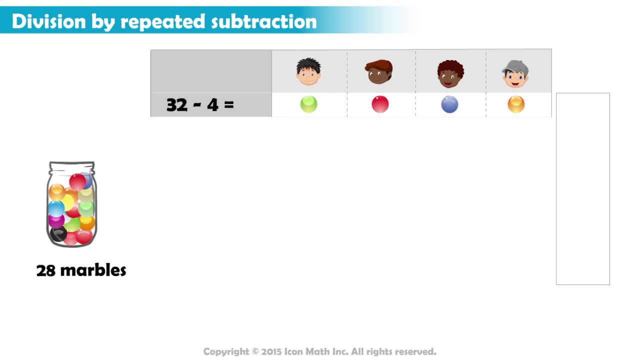 and we give each player one marble, Leaving us with 28 marbles. Across the margin, we write 1 to indicate that each player got one marble. Now we take another 4, and that leaves us with 24 marbles. 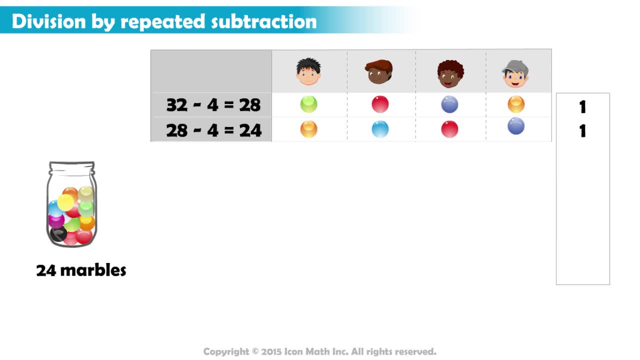 We also write 1 across the margin to show that every player got another 1 marble. Now we take another 4 marbles, leaving us with 20 marbles. Again, we note this with a 1 across the margin. 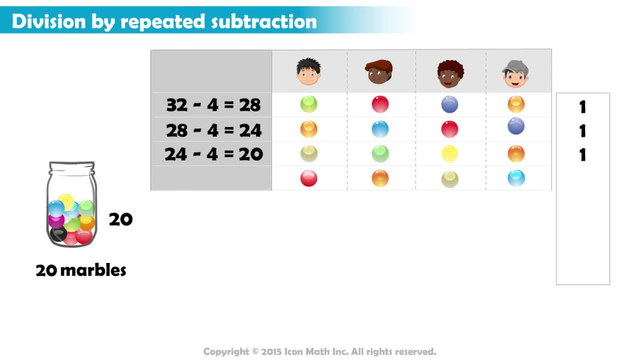 If we keep doing this repeated subtraction of 4 marbles from the remainder, while keeping a record of how many marbles we gave away, we will get a margin of how many marbles each player received. We will finally get to 4,. 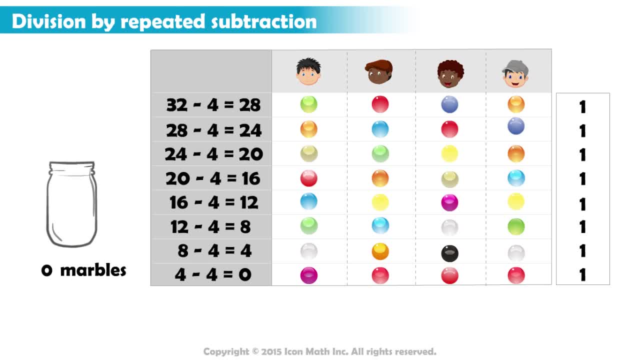 and 4 minus 4 is 0.. Since we reached 0,, this means we can equally split 32 marbles among 4 players without any marbles left behind. To find the answer of 32 divided by 4, we count the 1s we wrote in the marginal column. 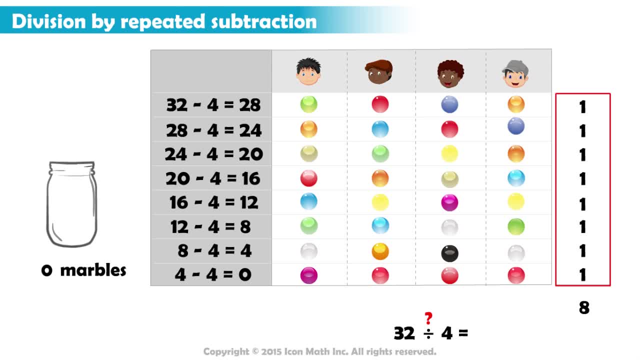 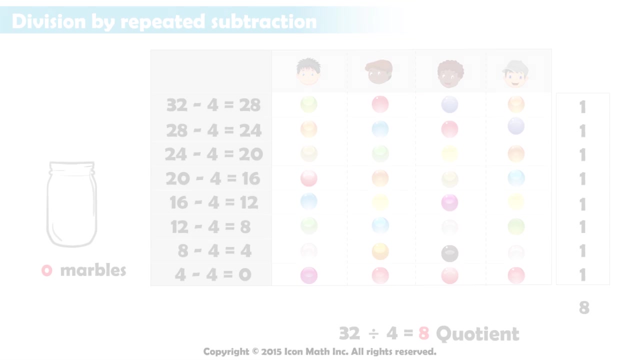 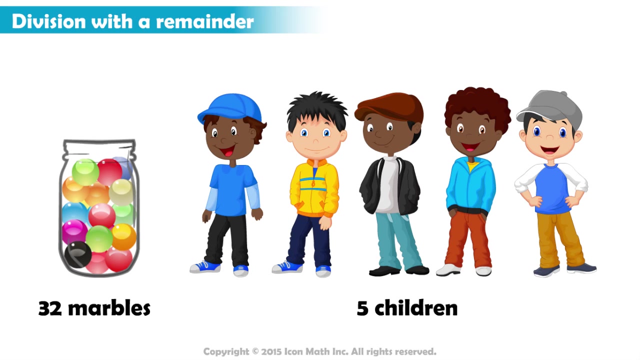 We have 8 1s, so the answer is 8.. Every player gets 8 marbles when we divide 32 marbles among 4 people, So 8 is the quotient Suppose. after 2 games, another one of Jim's friends joined them. 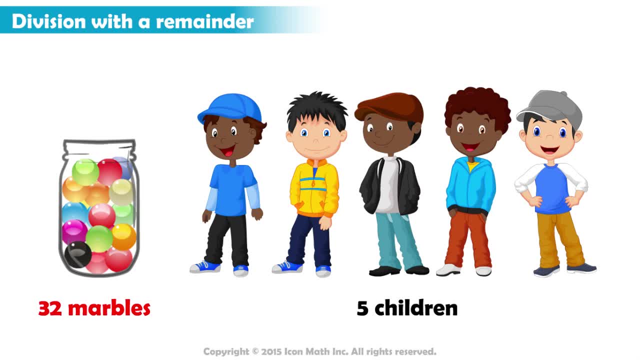 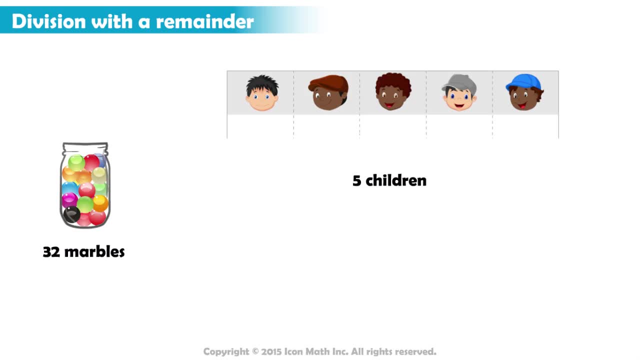 To play a new game. Jim has to divide 32 marbles among 5 people. Let us do the division using repeat. Let's do a repeated subtraction And leave a marginal column to the side to keep count of the number of times we gave marbles to the players. 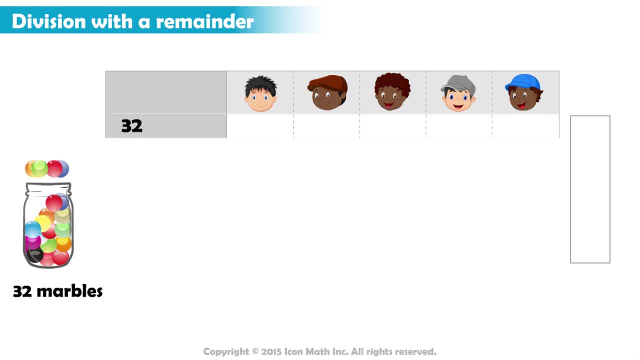 So we begin by taking away 5 marbles and giving each player 1 marble. This leaves us with 27 marbles And we write 1 in the marginal column to the right. This leaves us with 27 marbles And we write 1 in the marginal column to the right.